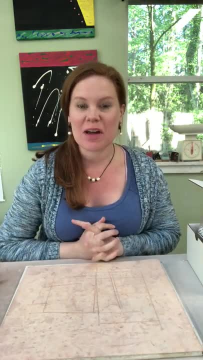 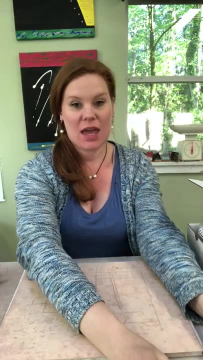 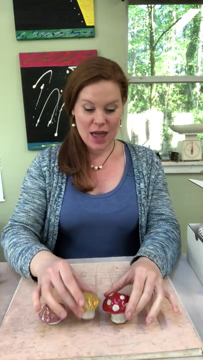 Hey, welcome back. This is Lisa Ingram, and today we are going to do our social distance pottery class number two, where we make these awesome mushrooms. So I'm so glad that you could be here today and, whether you are a kid or an adult, I 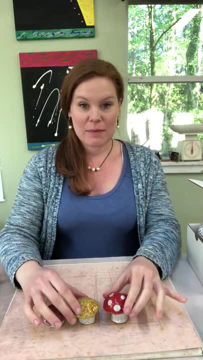 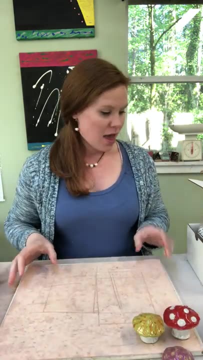 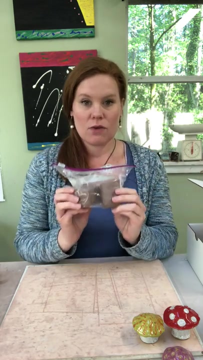 think that you will have a blast making these. So I'm gonna set these aside, maybe where you can see them just a little bit for your inspiration, and I'm going to show you what you have in your kit. So I've got two blocks of clay for making. 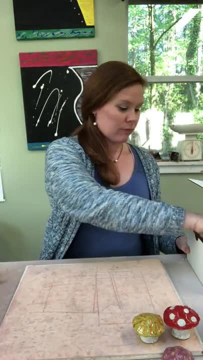 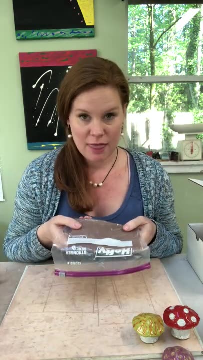 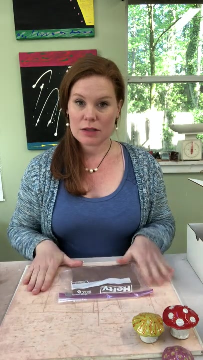 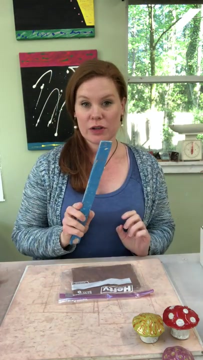 the mushroom caps, and then you'll have two baggies of slab clay and that is for the stem right here. So in addition to that, you'll want to have some kind of surface that you can work on, so you can take your box and open it up flat and work on top of that. A ruler is also very 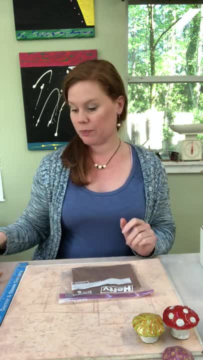 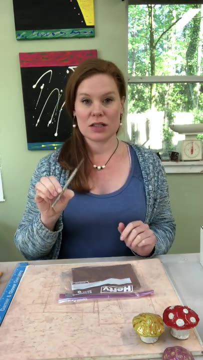 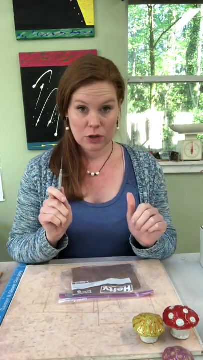 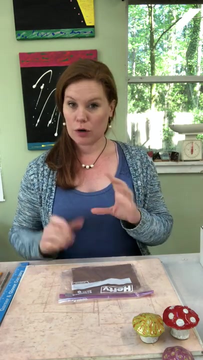 nice to have A paintbrush, A pair of scissors And something to scratch with, so I like to suggest a plastic fork, especially if you're a kid, because something pointy cannot feel good sometimes. So go ahead, pause the video and go and get your supplies um. a bucket of water or bowl of water is also really. 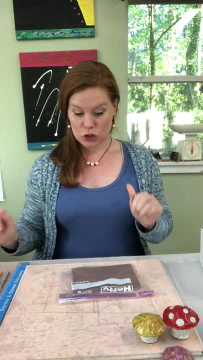 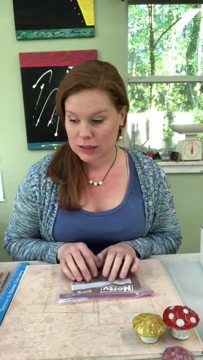 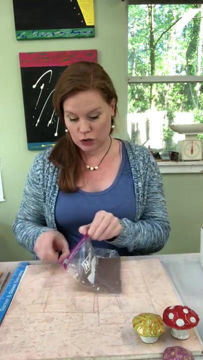 helpful. um, okay, so the first thing that we're going to do is we're going to get our clay out of the bag, our slab clay, and so you can unzip the bag and you can pull it straight out, or, if you feel like you're going to catch on the sides, you can use the scissors and cut your bag. 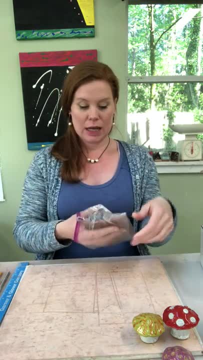 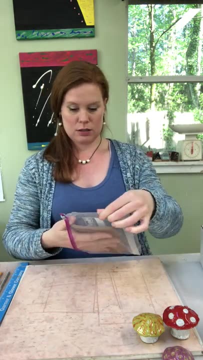 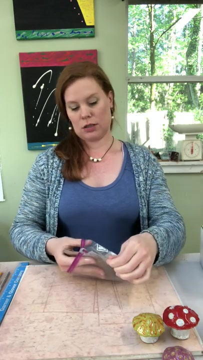 open, it doesn't matter. it might want to stick in there just a little bit. so be gentle as you release the clay and it will come out. mine kind of wants to catch on the side here, so i'm going to go corner kind of work it out. scissors are also fine. they make it easy. 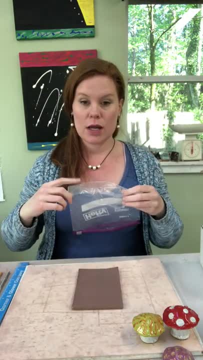 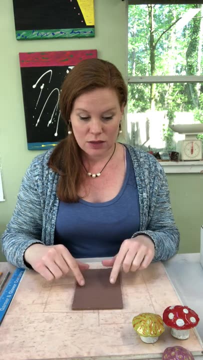 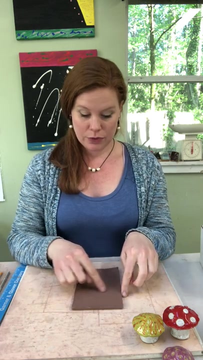 okay, so there's my clay and this is a four inch by six inch piece of clay. so you're going to get your three stems out of this piece of clay. so if you want all of your mushrooms to be the same height, you would cut three, two inch tall pieces of clay if you want. 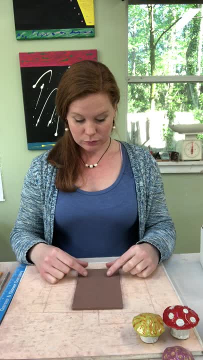 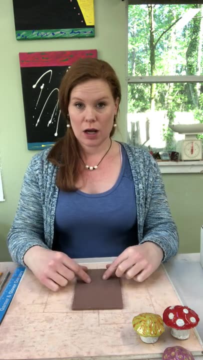 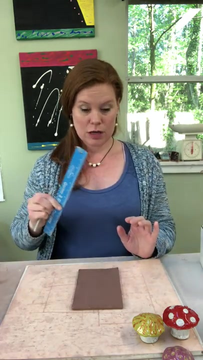 them to be different heights. then you could do a one inch, a one and a half and a two inch, or a two and a half, a one and one and a half. um, you can kind of eyeball it. you don't have to use your measuring your, your ruler or your measuring tape or your measuring stick. 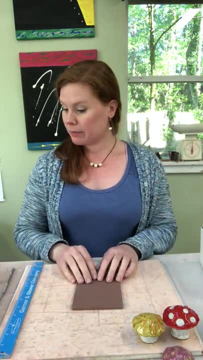 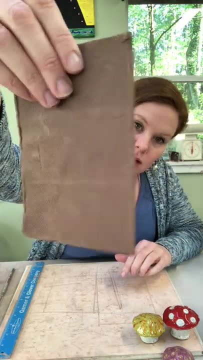 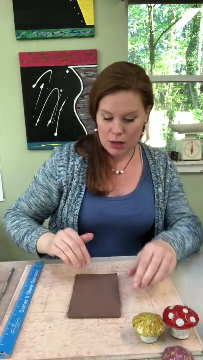 but just think about how you want it to look, um, so the first thing that we're going to do is we're going to smooth out this clay because, if you can see, it has a little bit of a canvas texture on it and that it comes from where i use the slab roller, which is a piece of equipment. 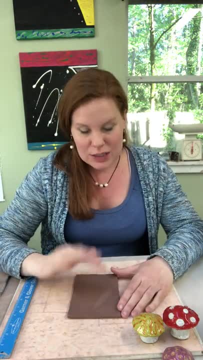 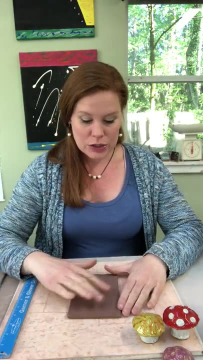 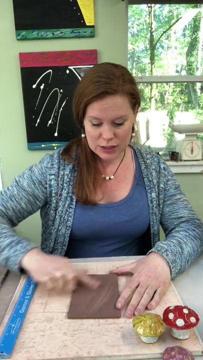 in my studio to make flat pieces of clay. so instead of having to use a rolling pin, i have a machine that i roll it through and it makes flat pieces of clay for me. so, anyhow, i'm just going to take my finger and i'm gonna rub, very gently rub out this texture. so i'm working. 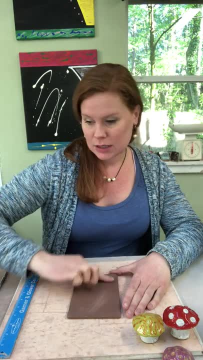 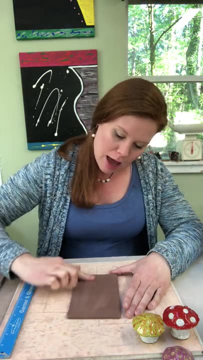 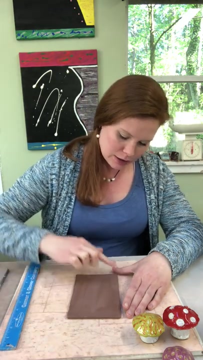 hard not to change the shape of the piece of clay. i could press really hard and it would change the shape of the clay. i'm just swiping the surface. it doesn't have to be perfect. i just want to get it a more smooth than it already is. If you have something like a gift card, that's. 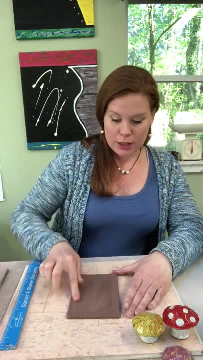 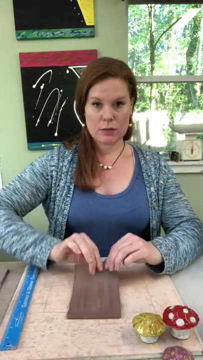 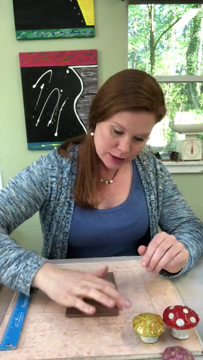 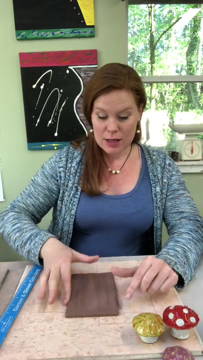 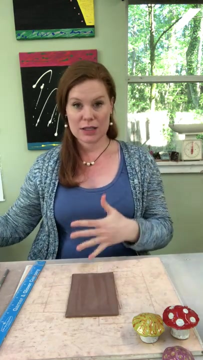 also a really good option for smoothing out your clay. So that looks pretty good to me. Give you a look at that. So today we are going to make one mushroom, together with the spots on top, and then you can make the rest at your leisure and use your own creativity, But the same steps will 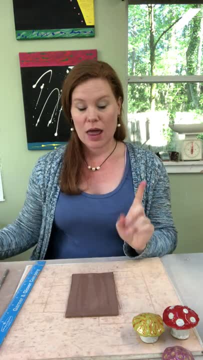 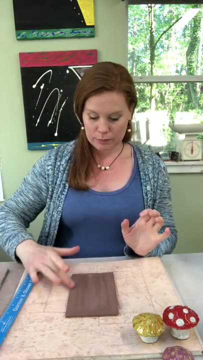 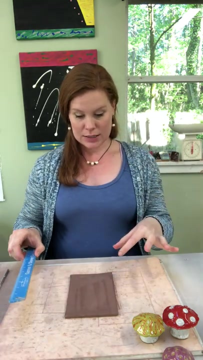 apply. and this is video part one, and then I'll do a video part two where we add the glaze to these. So that's going to be a really fun step as well. So I'm going to start with making a two inch slice of this clay here. So I'm going to take my ruler, I'm going to lay it on. 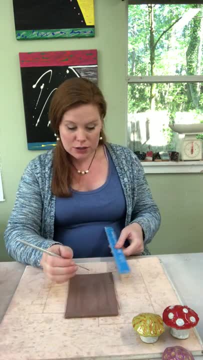 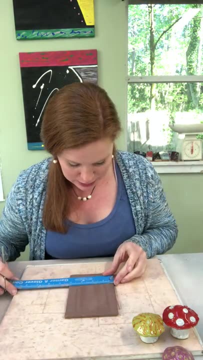 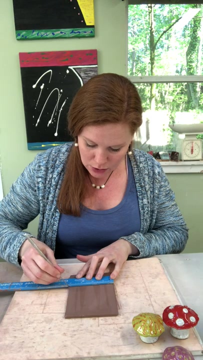 here, I'm going to make a little mark at two inches on the left side, and then I'll make a mark at two inches on the right side, And then I'm going to connect those lines with my ruler and I'm going to make a cut all the way through, And so I 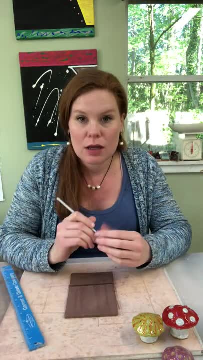 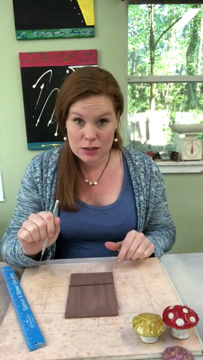 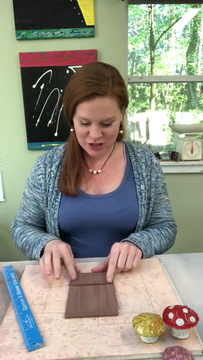 didn't mention this before, but what you can use is a plastic knife. I'll put that in the comments, That a plastic knife is really good for making these cuts, or also a toothpick is really good for making these cuts. So I apologize, I forgot to add that earlier. 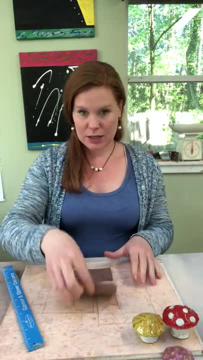 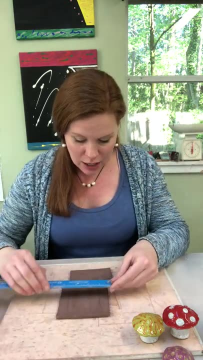 Okay, so the next step is I'm going to set this little piece of clay aside. This is going to be for the other stems, And actually I'll just show you how I'm going to cut these. I want these to be different sizes. 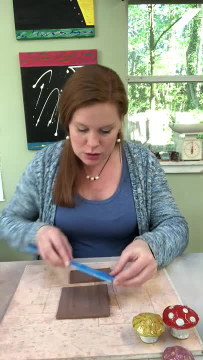 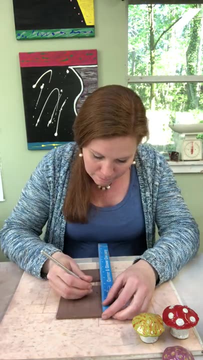 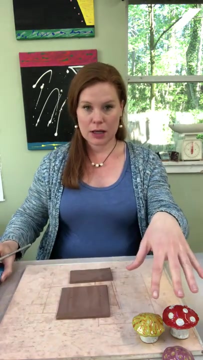 So I have a two inch, I'm going to make a two and a half inch and that'll leave me with a one and a half inch, And then I'll have three different sizes. So if you like the stair step, look like I did with this set. those are good measurements for 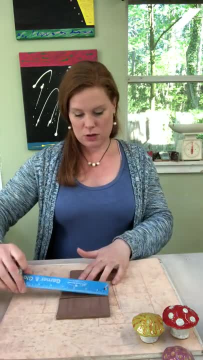 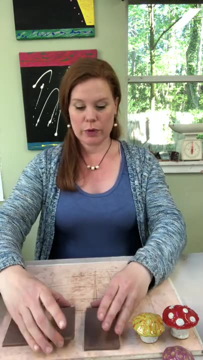 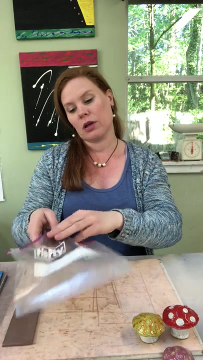 you. So two inches, one and a half and two and a half, So I'll have three different size stems like that. So we'll work with the two and a half And you can always set these back in your bag while you work, or if you cut your bag open you can lay it. 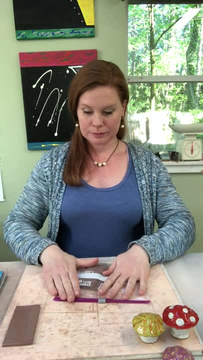 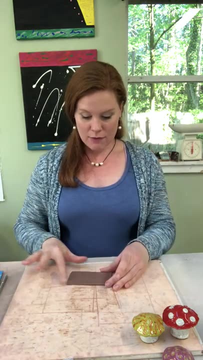 on top, and then they'll stay nice and soft for when you're ready to work with them. So we have our little rectangle right here, our first little stem, And so what I'm going to do- and watch first before you jump- is I'm going to cut this. 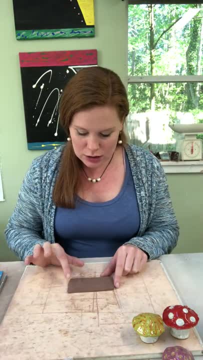 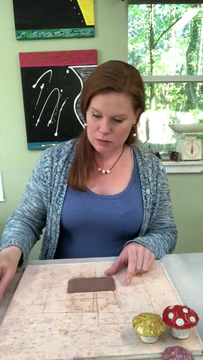 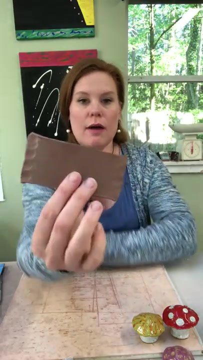 out and I'm going to take my finger and I'm going to gently smush the edge. So I'm going to do that on both sides. I'm only coming in about a third of an inch And I smooshed both sides So it looks like this. It just flattened those sides out a little. 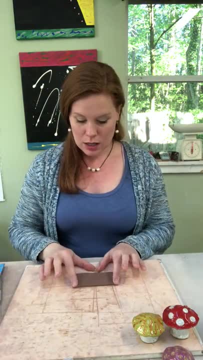 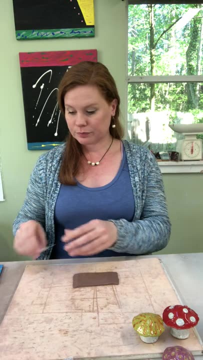 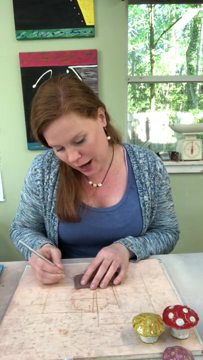 bit. You can go ahead and do that And just be careful not to over smush it. And then what I'm going to do is you'll take your toothpick or your plastic fork- whatever scratching tool you have- and you're going to scratch where you. 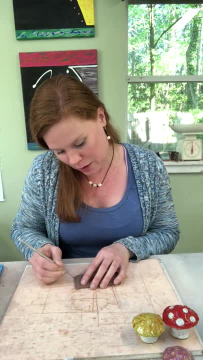 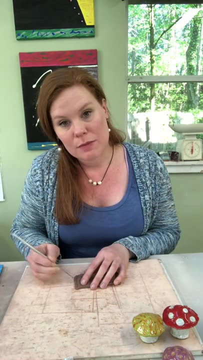 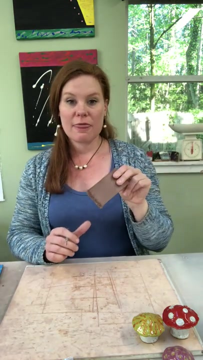 smooshed it on only one side For now, And this is called scoring, And this just opens up the surface of the clay because we're going to wrap it around and stick it to the other side. So that's what my scratching looks like, And then I'm going. 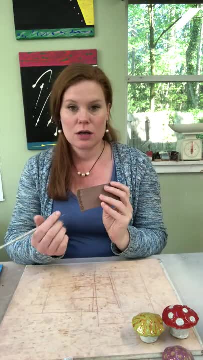 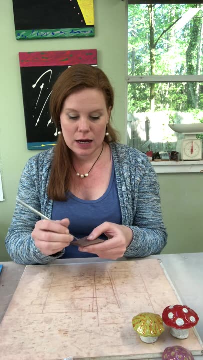 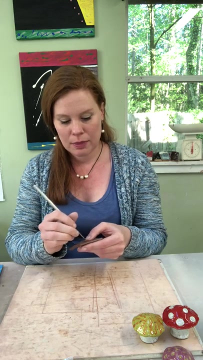 to scratch on the back on the opposite side. So I'm not scratching on the same side here. I'm going to go to the other side and scratch on the back And again, I'm only going in about a third of an inch And my scratches are fairly shallow. 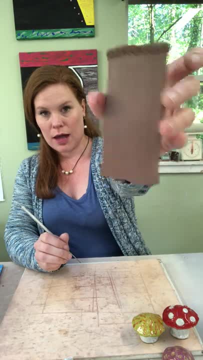 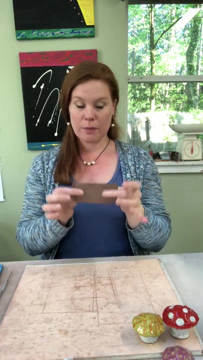 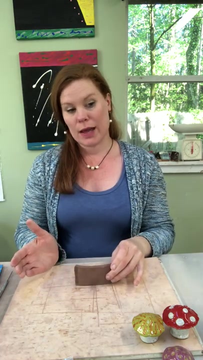 And so they look like this on the back and this on the front. So now you have two sides that are scored. You can pause this at any time. You don't have to keep up with me and take this at your own pace. That's my. 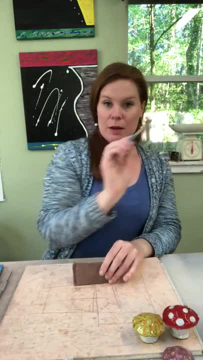 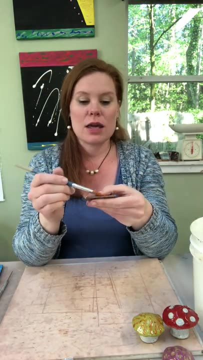 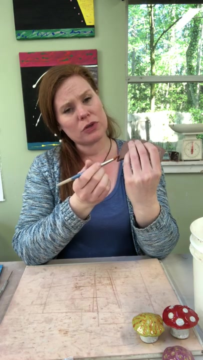 advice to you. So now I've got my paintbrush, I dipped it in my little handy water bucket that I have right here, And I'm going to wet here where I scored the clay. This clay is nice and soft, but I'm just going to go ahead and wet both of 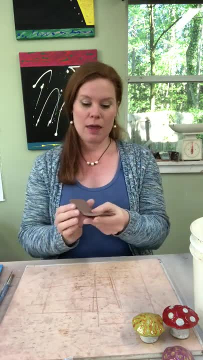 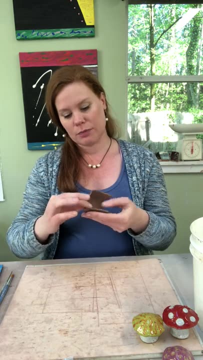 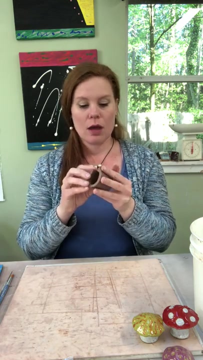 those scored edges to make it extra sticky. And now I'm going to gently just wrap it around. I'm trying to mold the clay a little bit because if you wrap it too quickly it might crack on you. I'm just going to slowly wrap it. 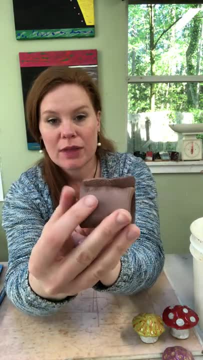 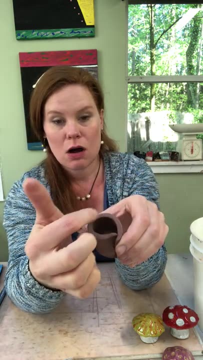 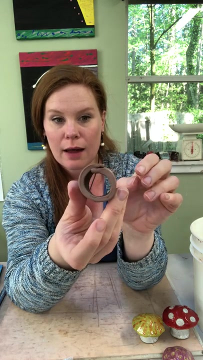 around, And then I'm going to overlap that third of a clay on both sides, because what we want to make is an even thickness all of the way around. So you don't want to have a very thin edge right there, You want it to overlap enough that you're making a good thick bond, right? 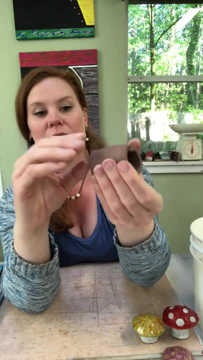 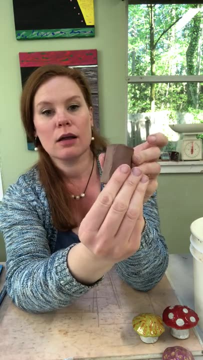 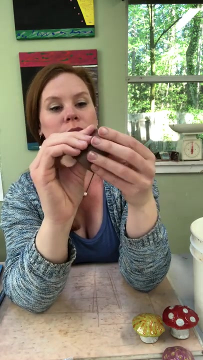 here, And then we're going to add some pressure, gentle pressure, to press it together. So I've got one thumb on the inside and a few fingers on the outside. I'm just pressing it together. I'm not going to worry about making these seams. 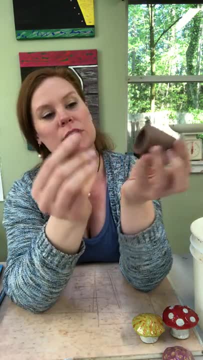 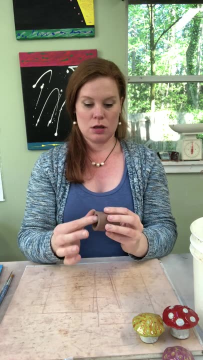 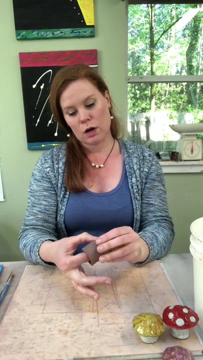 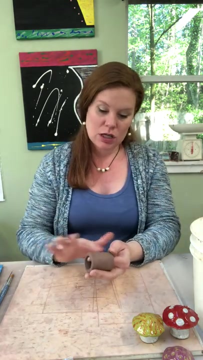 disappear, But I am going to smooth it. So on the bottom I'm going to smooth it with my fingers And then here I can smooth my thumbs a little bit, A little bit of that water squeezed out, and that's okay. You can use just a tiny bit of water to help you. 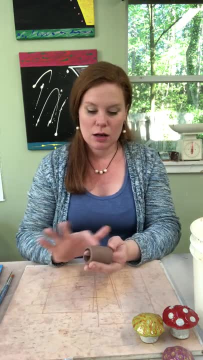 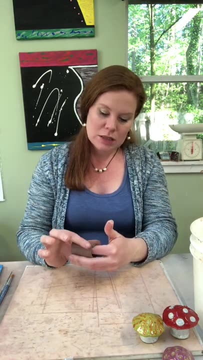 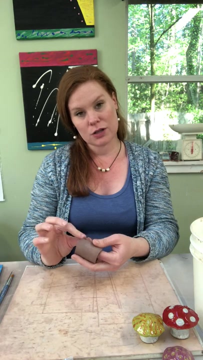 smooth. If you use too much, it gets muddy and it's going to want to fall apart on you, Which is not always the case and I won't be using this Once again. I said: just be gentle with your clay. It's better to do it slowly and not Connapt. 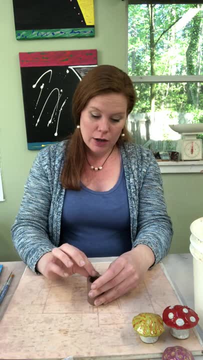 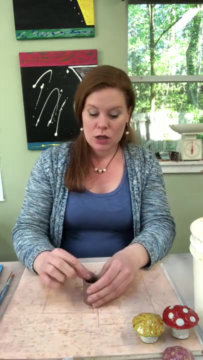 collopse your clay than to try to rush and it crack and fall apart. If, for some reason, it does fall apart, you can get a rolling pin of your own and roll it back out and just go for a similar thickness to your slab. 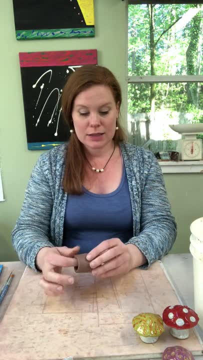 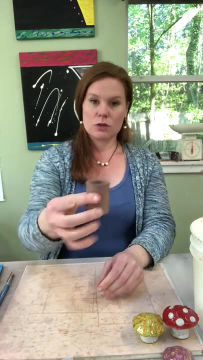 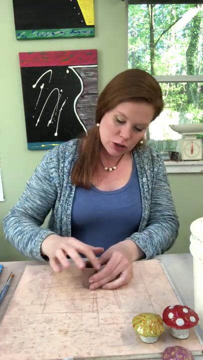 start over. So just keep that in mind. It's best to work slowly so that you don't run into any issues. Okay, so there's my little two inch stem and if you have any little cracks that start to form on the edge- sometimes you'll get little cracks from stretching it. You can get one just. 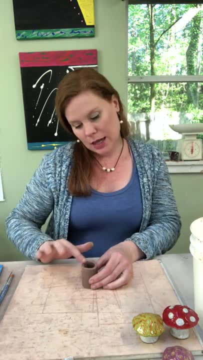 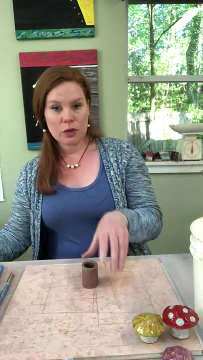 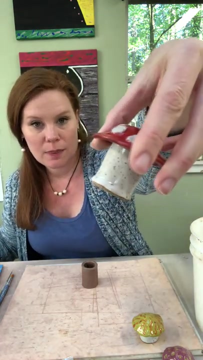 one little finger of water and work it around that rim right there. So this clay is brown, and the cool thing about this clay is it has speckles in it, and so that's one of the reasons why I wanted to use this clay for this project. But you can see, this mushroom has some speckles. 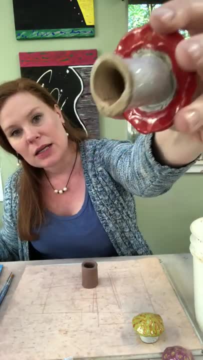 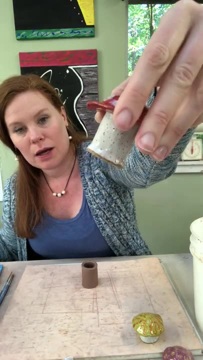 showing through the glaze So you can see it also has speckles on the bare clay, but they're really fun poking through on the top And on the side here. So just because the clay is brown doesn't mean that the glaze isn't going to. 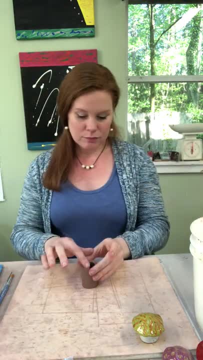 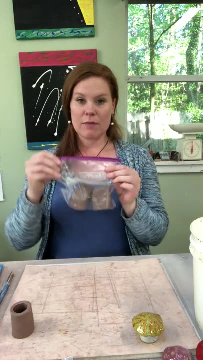 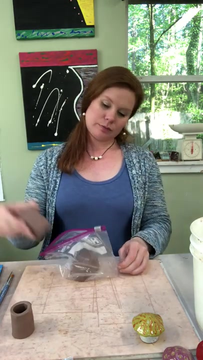 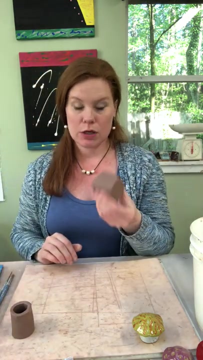 make a big difference. So that's, that's your stem, right here. I'm gonna set it aside. and then I have my bag of clay here. I'm gonna get out one chunk of clay and this is enough clay for three mushroom capsules. So I'm gonna get out one chunk of clay and this is enough clay for three mushroom capsules. 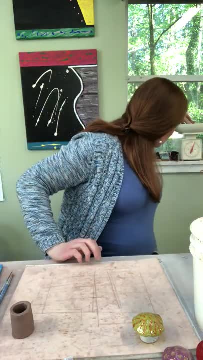 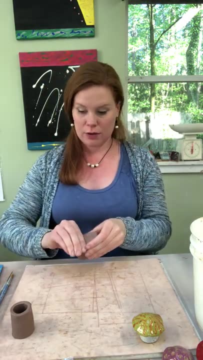 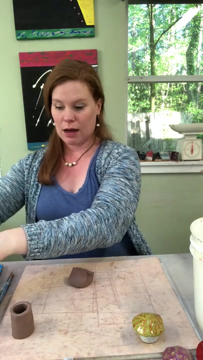 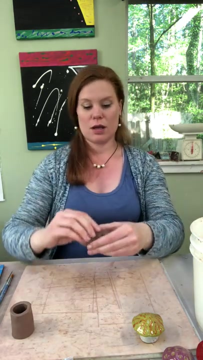 So it's about like a little less than half a pound and I'm just gonna pinch off a third of this clay. I'm gonna put the rest back in my baggie because, again, anytime we get clay out in the air it's going to change on us. It's gonna lose its water slowly, but it's a lot nicer to work with nice soft clay. 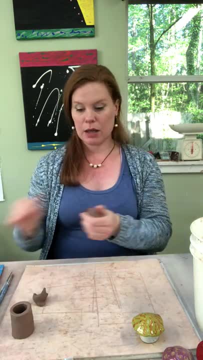 Since this is brown, I'm going to go ahead and add a little bit of brown to the bottom. Since this is brown, I'm going to go ahead and add a little bit of brown to the bottom. So this is my medium mushroom cap. I'm going to pinch just a little bit of this off. 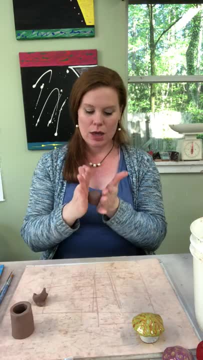 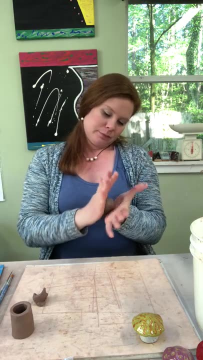 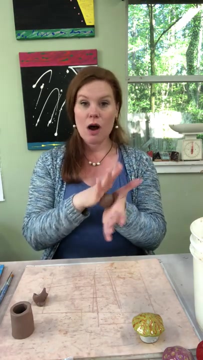 I'm going to roll it into a ball, So I want to start with just a little ball before I make my pinch pot. And so if you did the last project where we did turtles, you know all about pinch pots, And so we're going to shape this completely with our hands. 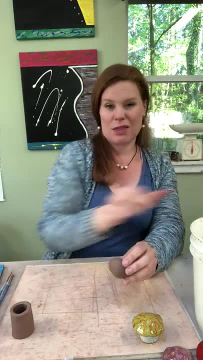 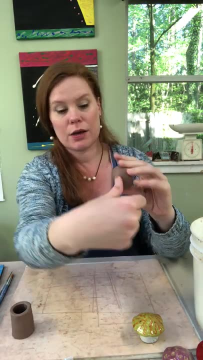 And you'll start with a ball- the ball. Then I'm going to get my thumb just a little bit wet in that bowl of water and then I'm going to find the middle spot in the bottom right here and I'm going to work my thumb into it. So 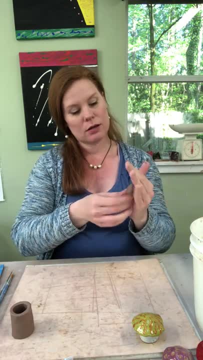 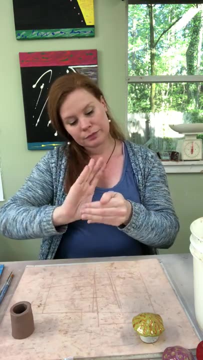 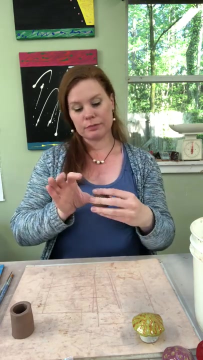 I'm supporting the clay with the opposite hand. I'm going to work the thumb in. I don't want to work it all the way through, I just want to work it in a little bit until I feel like I'm getting close to all the way through, but not about to go through the top. So it's going to look like this: 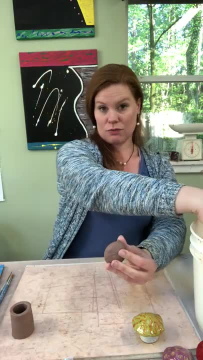 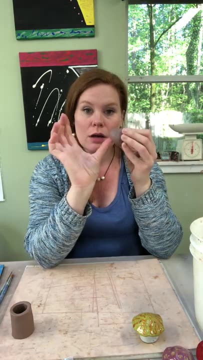 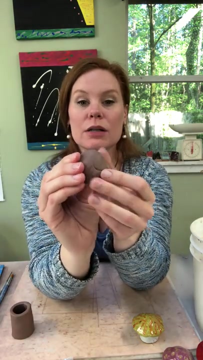 It'll start to look like a mushroom top and then I just need to rinse my fingers off there. Now I'm going to start to pinch it. So I'm going to pinch like this: one thumb on the inside, these fingers on the outside, I'm going to start at the top and I'm just going to twist and pinch and this thins out. 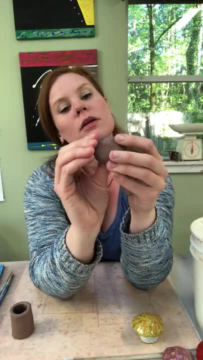 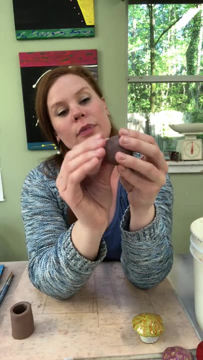 the clay and it's going to make it grow. Don't worry too much about the shape right now, because we can change that. I like to smooth it a little bit as I go, but we'll do that. We'll do more of that towards the end. 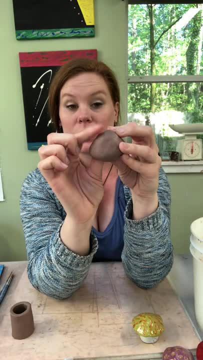 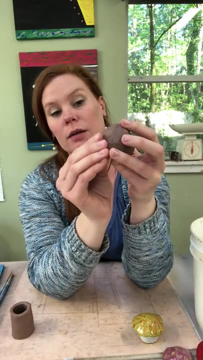 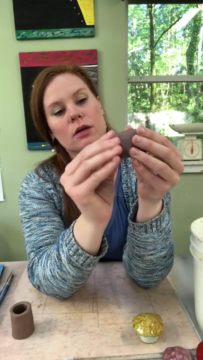 So I'm just turning and pinching, and I started here. This is the top of the mushroom cap, so I start at the top and, as I'm pinching all the way around, I'm working towards the bottom, Which is this rim of the clay, the most open part, and so I'm seeing a little bit of cracking here. 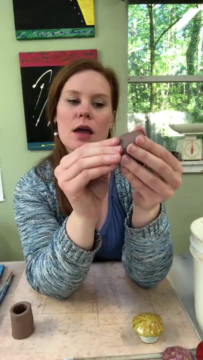 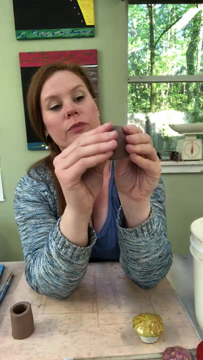 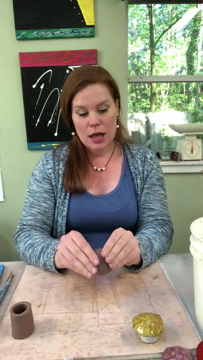 but, lucky for us, mushrooms kind of look like that at the bottom, So we can rub some water on it to get rid of those cracks, or we can keep them. It's really up to you. but they're pretty easy to get rid of. So now I've got both thumbs in there and I'm just turning and I'm twisting. 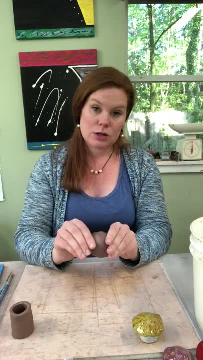 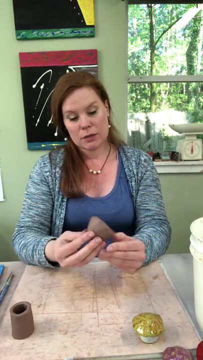 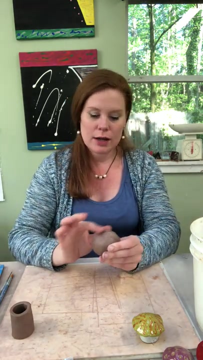 everything my outside fingers are smoothing. we're just making this little upside down bowl. so right side up it's a bowl, upside down it's a mushroom cap. i'm going to get a little bit of water and rub it on here to get rid of some of these cracks, because what i want to do now is 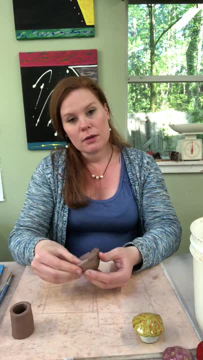 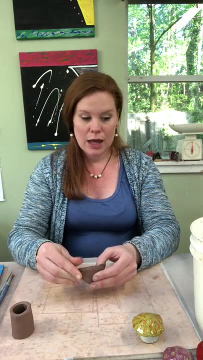 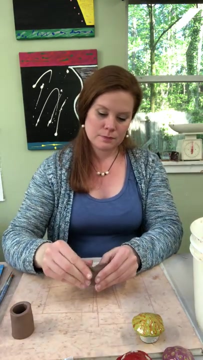 i'm going to flare out the rim, so my thumb is just smoothing that clay outwards, and this is opening up the bowl or the mushroom cap, so it's going to get more of an edge like this one. i'm not squeezing it really hard. this is all going just a little bit at a time and every so often 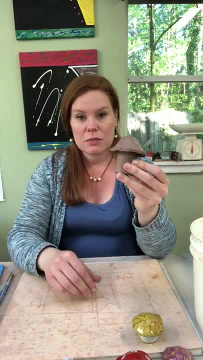 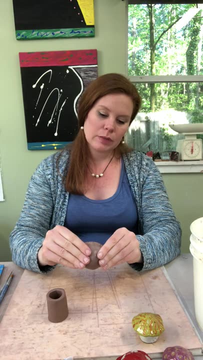 it's a good idea to hold it up to your stem to see what it looks like. you don't want to make the edges razor sharp because they are going to be very hard to hold. because they are going to be very hard to hold because they are. 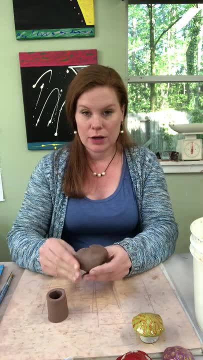 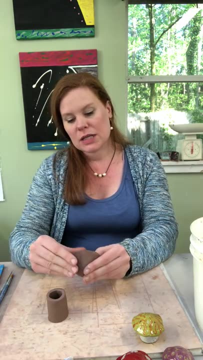 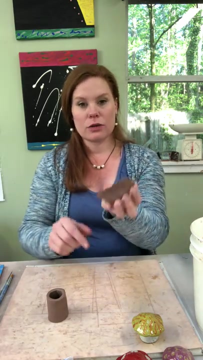 going to get very hard in the kiln and you don't want it to be very fragile or so pointy that it can scratch you or cut you when it comes out. So I'm going to go back around this rim and just smooth it. I like these little uneven edges because it really looks like the real thing. 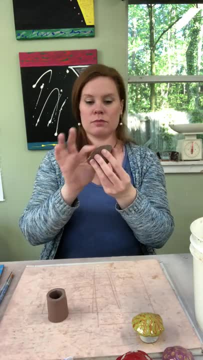 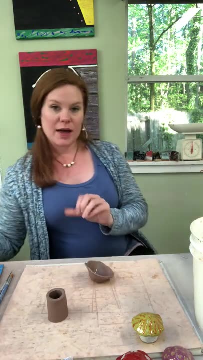 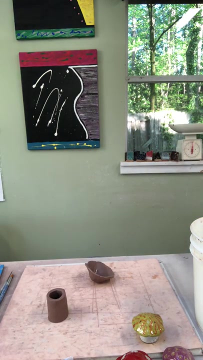 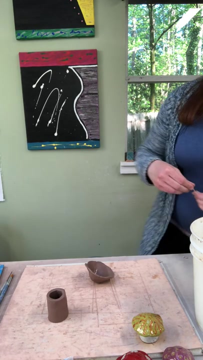 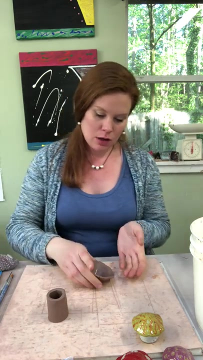 And now, if you have a toothpick, I'm going to grab one. I think I've got one over here. There's some designs you can do, toothpicks that are really cool. All right, Okay, so this is an optional design that you can do, but I'm going to support it in my hand, like: 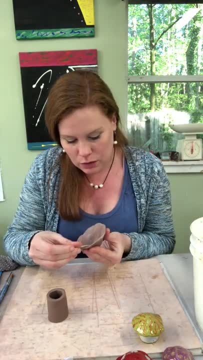 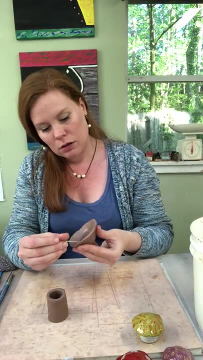 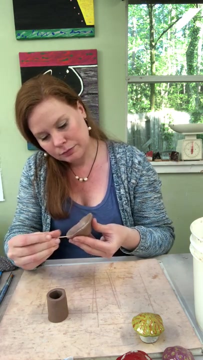 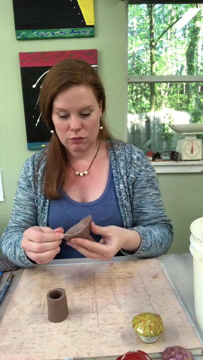 this and take my little toothpick and I'm just going to make a little line here, Just like that. I'm not cutting, I'm just slowly making a little line, I'm going to rub the clay off And then I'm going to work this around to give it that underneath ridge effect. 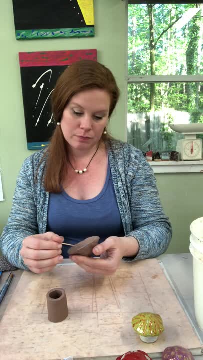 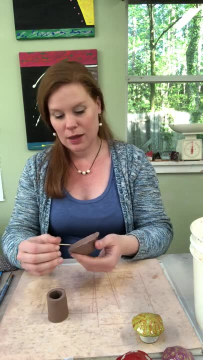 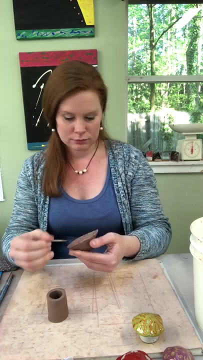 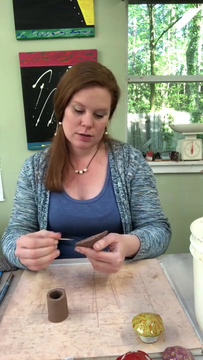 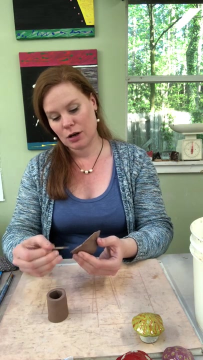 You can kind of rock it or you can pull it, But I love how intricate Mushrooms are and how they do have designs underneath them, And so we can make ours look like that. I like doing these nature projects because, good one, You have a lot of creativity that you can put into it, since things in nature 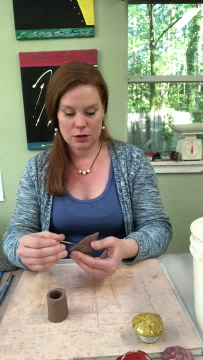 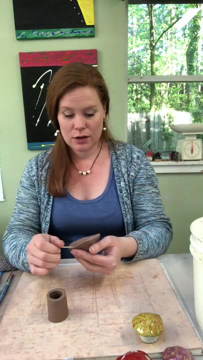 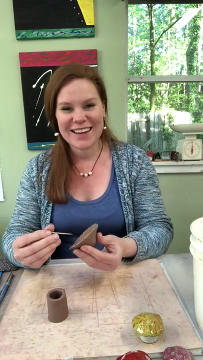 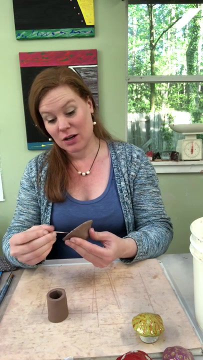 just come in. so many different shapes, so many different patterns, so many different patterns. So that gives us some really nice details, different colors, and it's just fun to celebrate spring when things are so different. Some things are still the same, like mushrooms and flowers and the weather going from warm to cold on a daily basis. 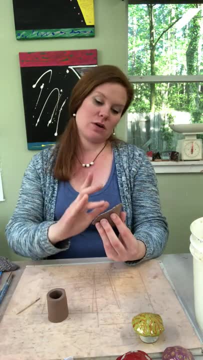 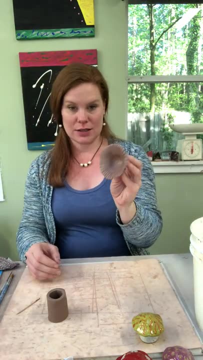 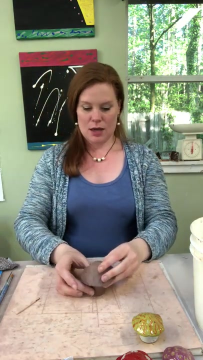 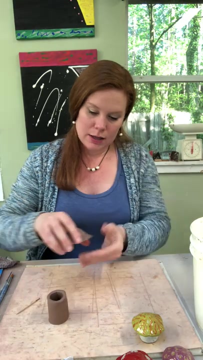 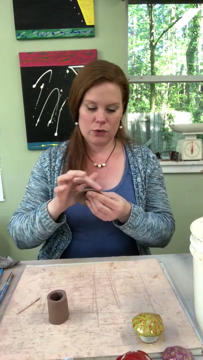 and tornadoes and thunderstorms and all that are pretty normal. So there's my little underneath design. Who knows if anyone is gonna see that? So it's gonna look like this and I'm gonna smooth the top a little bit And now that I know I've got this design underneath, I'm being really careful, not 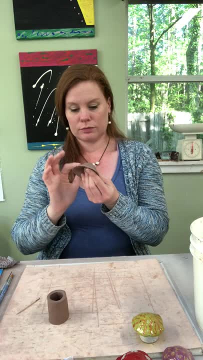 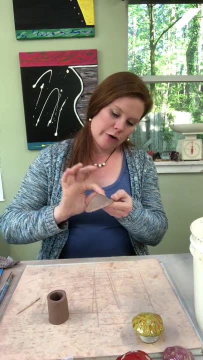 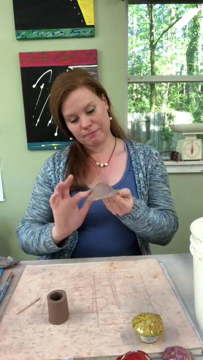 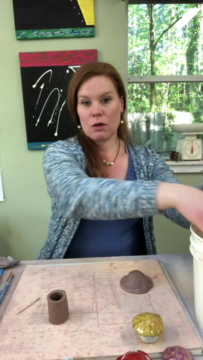 to disturb that design And, like I said, I don't have to get this perfectly smooth. Mushrooms are so unique, they've got so many different looks to them. I'm gonna leave some of it a little bit organic looking. So I'm gonna set this down and now we're going to attach. 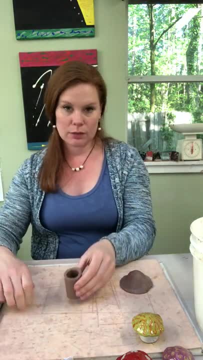 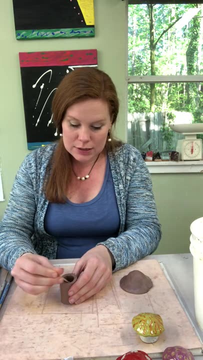 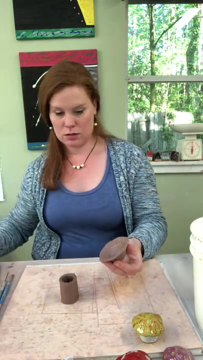 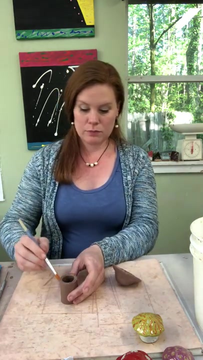 these So you can use your toothpick. since I've got one now, I'll use that to score the top. So I'm gonna take the top of the mushroom stem and then- this is my little trick- I'm gonna put a little bit of water on the mushroom stem. I'm going to score it just a little bit more. 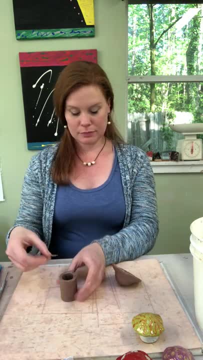 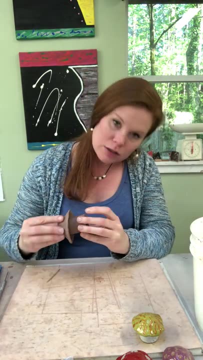 This is making it muddy, Then I'm gonna take my mushroom, I'm gonna set it in here and I'm going to put my mushroom in here and just kind of give it a wiggle. Mine's a little bit lopsided, so I'm gonna. 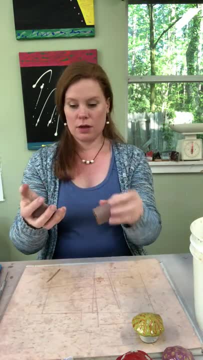 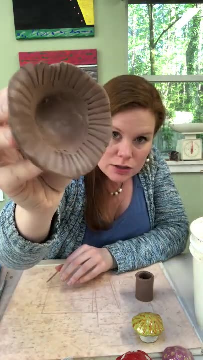 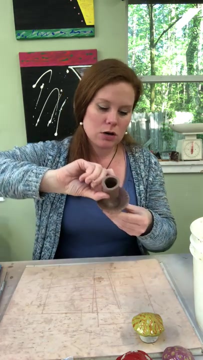 adjust that, Then I'm gonna pull the top back off and I'm gonna see where that mud ended up. So I have a circle of mud in there and if you don't, you can also, when you have this on here, just make some marks with your toothpick as to 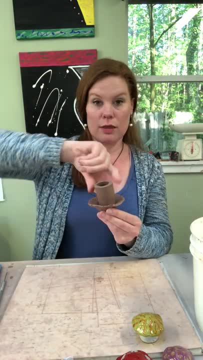 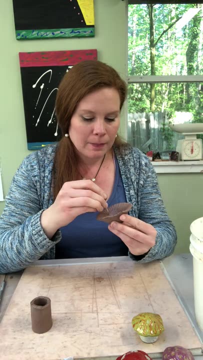 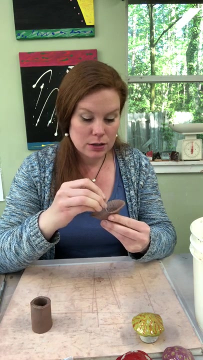 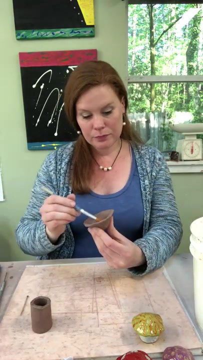 where the clay meets, so that you know you score on the inside of that line, And then you'll just score here, And that's gonna make a really good place for these two things to bond to one another. Okay, so I'm gonna add my water on the inside now. 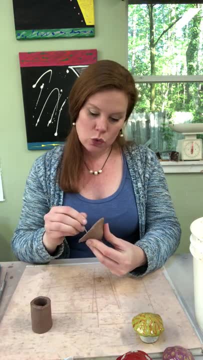 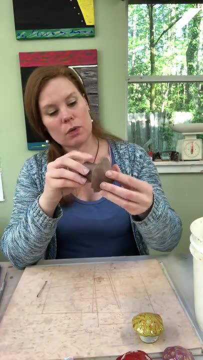 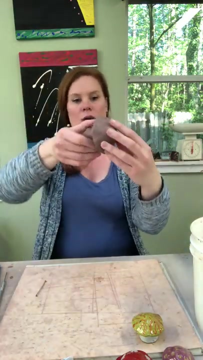 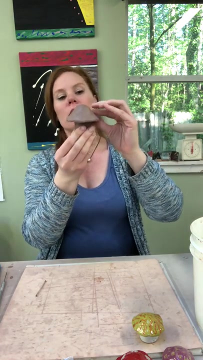 I'm gonna re-score it just to be safe, and now I'm going to attach. So again, I just kind of wiggle it on there. If it looks a little lopsided, just wiggle it until you're happy, and then we can still even adjust this. 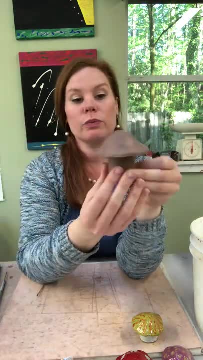 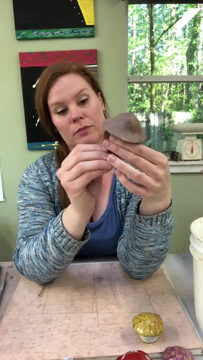 And then I'm just gonna fold it down so it looks very mushroomy On my others. don't drop it. like I just did On my others. I kind of fanned out the bottom so that they wouldn't be so tipsy. This one doesn't build tipsy, It feels pretty. 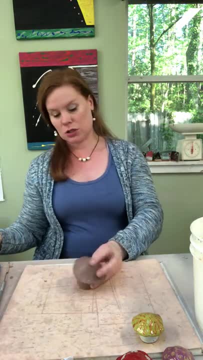 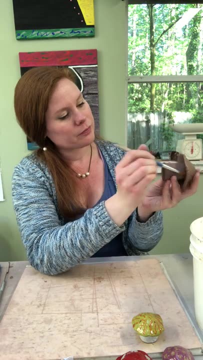 sturdy. so that's just an option. And then you can use your paintbrush, making sure your lid doesn't fall off, and smooth out that seam in here, just to make it nice and neat. I just love to do it in this size. This is what I love to do, And then I'm gonna see how that looks. 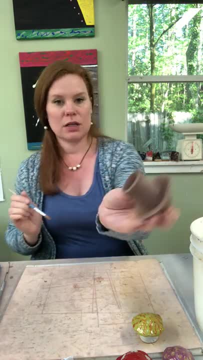 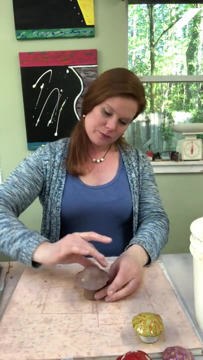 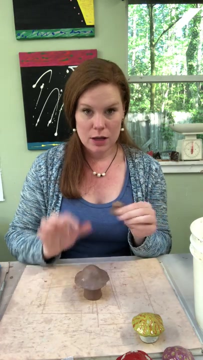 I just love this design with the toothpick when you hold it upside down. That's so fun. Okay, it's like a little surprise, Okay. so now I've got my little extra piece of clay here, I'm going to make the spots for the top. 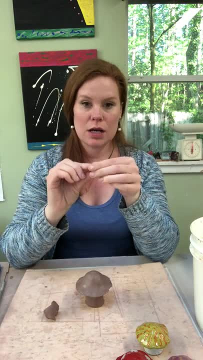 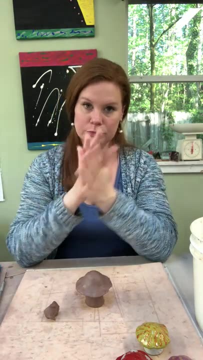 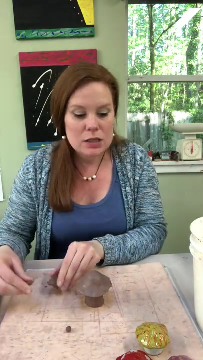 So I'm just going to pull off a tiny piece of clay and I'm going to roll it in my hand. So he's very rolly and you can do. um, let's see, this one's got seven dots. You can do all your dots at once, so they're about the same size, or you can do them. 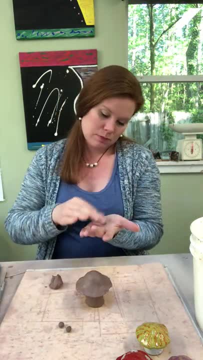 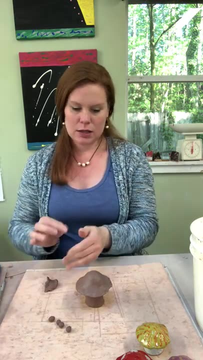 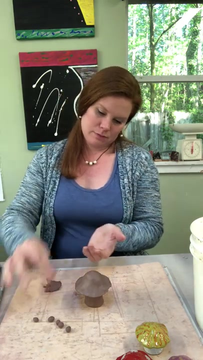 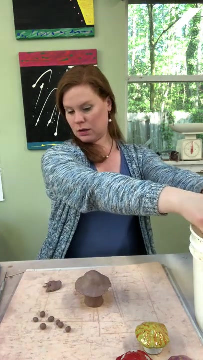 one at a time and then attach. So they're really. they don't take long to roll and they don't have to all be the same size. They can be various sizes. So there's seven of mine, and then- this is the fun part- you get to squish them. 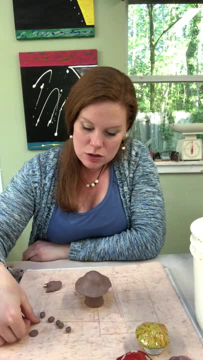 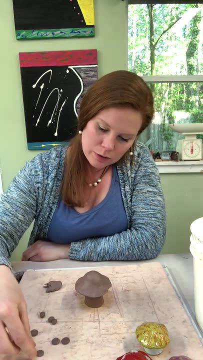 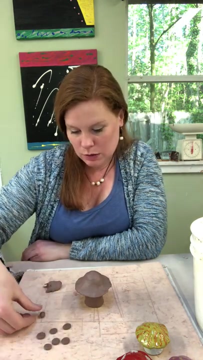 So I'm just going to use my thumb and squish them down. You can just squish them right down on your cardboard. You don't want them too flat. They start to crack when you flatten them. But, like I said, that's okay. They're just funky little mushrooms that we found outside. 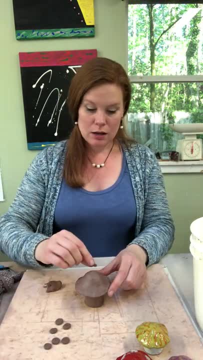 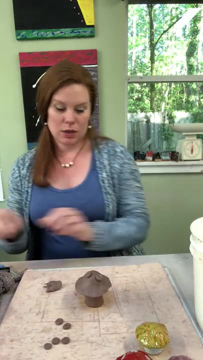 I'm going to decorate my yard with mine, So then you can place them all on here, or you can stick them on and then decide where you want them to go. I don't think these are all going to stick if I stick them all on right now, But guess what we're going to do. 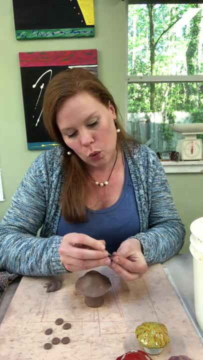 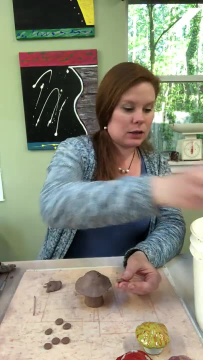 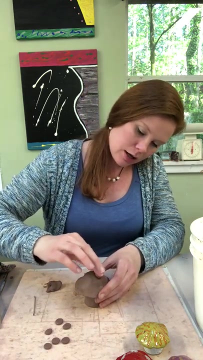 We're going to use our little toothpick, We're going to score And we're going to score the mushroom and then I'm going to add a little bit of water. I'm not going to have to be as careful with these because they're not supporting a mushroom cap. 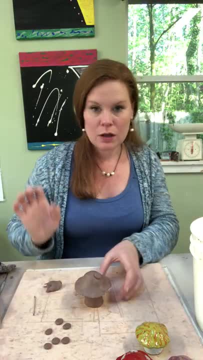 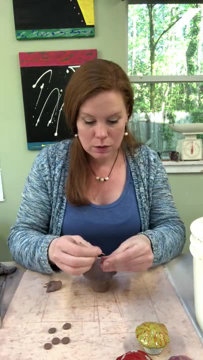 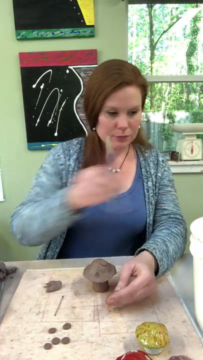 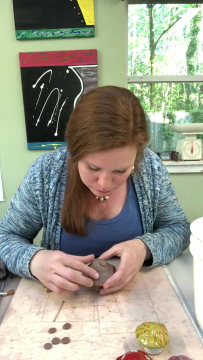 Then I'm just going to tap it on down there, So there's one little dot and then I can do another one. I think I'll put him over here. Get a little more water. That's a little too much, Press it on. 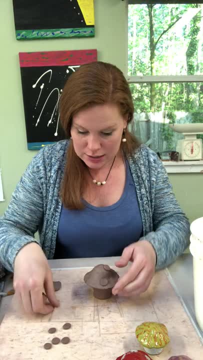 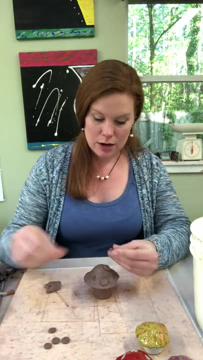 Okay, so there's two. He's starting to look very mushroomy and now you don't have to do dots. This is just an example of design. So now that we're at the dot and the remember, you can go to your dot and dot, You can. 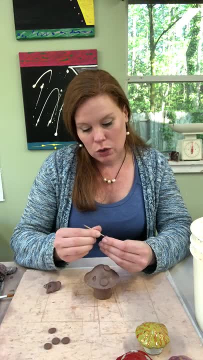 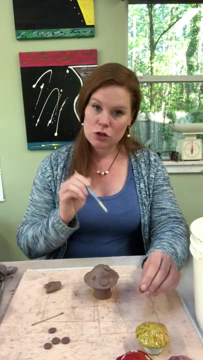 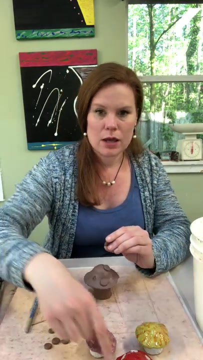 design part. this is where you get to get creative. so on this yellow one right here, I just did squiggles. I took the tip of a paintbrush and drug it through the clay to make little squiggles. then on the purple one, on the purple one right. 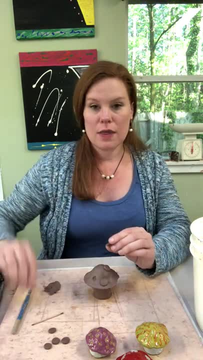 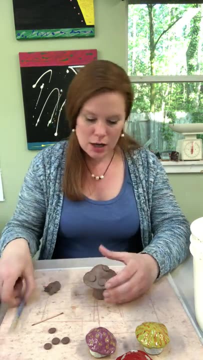 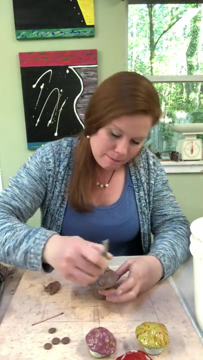 here I took the paintbrush and did dots and then I painted those dots inside the dots a different color. so there's all kinds of things you can do. I'm sure that you can come up with way more than that if you want to, if you get little cracks. 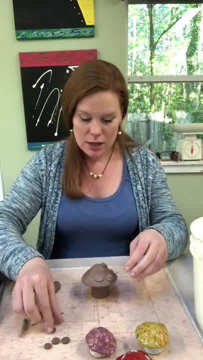 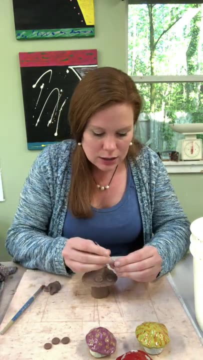 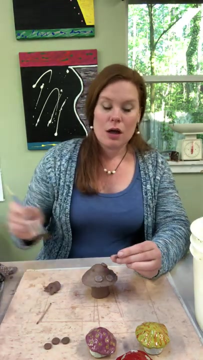 like I'm getting in the dots. you can wipe them with a paintbrush and they usually go away. but I wanted to show you guys the dots because this is one design element that does involve the score and slip method and you could just press it on and they would stay for a little while, but they would eventually fall off. 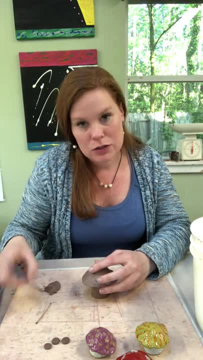 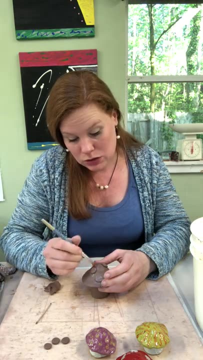 as the piece dries and goes away, and then they would go through the firings. it wouldn't be strong enough to hold. so I like to tell my students: whenever you attach clay to clay, you always score and slip. so that's a really good rule of thumb. but if you're carving, 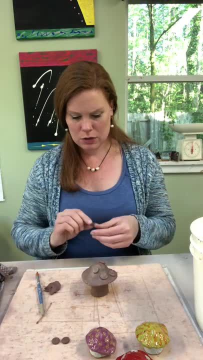 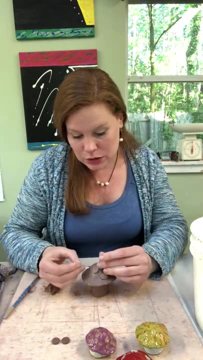 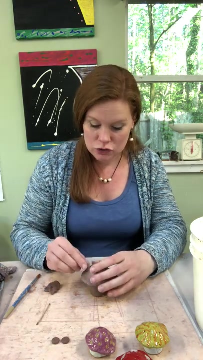 or dotting you don't? there's no need for that, so I can't wait to see what designs you guys come up with. after you finish your design, you can move on to the next one for art, to your next mushrooms, and then you're going to let these dry, so you want these. 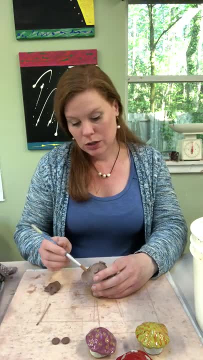 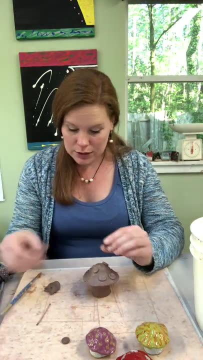 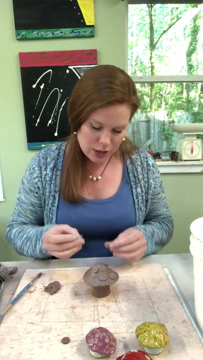 to dry for a few hours before you do your glazing, so you can go ahead and watch the glaze video part two, just so you see what we're going to do and get an idea of it. and then, after these harden up a little bit, we like to call: 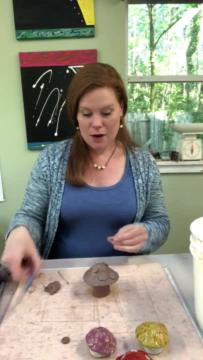 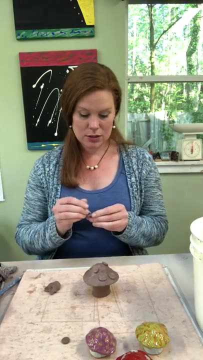 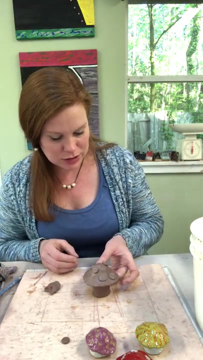 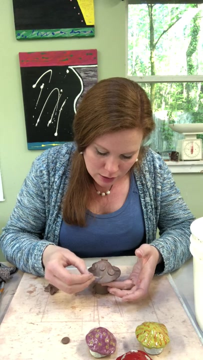 them leather hard when they haven't changed color yet, but they are not bendable anymore. when they're at that nice leather hard stage, that's a really good time to go ahead and do your glazing. so I've got one more spot to put on. let's put him over here, right where you can see it, and then we're gonna call. 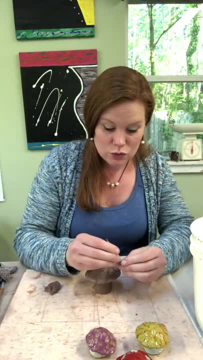 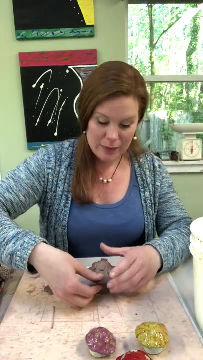 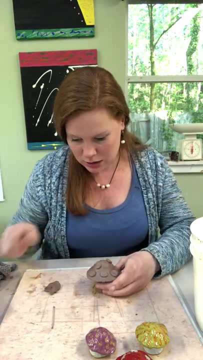 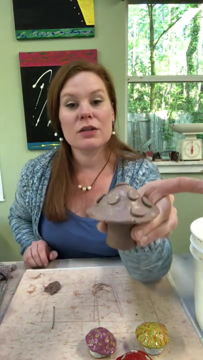 this guy done and you can go on and enjoy your other mascaras, mushrooms, creating your other mushrooms, and you can just rewind this video or back it up and watch any parts over that. you need to think I squished some of my underneath design. I'm gonna have to go back and fix it. so there's my little guy. 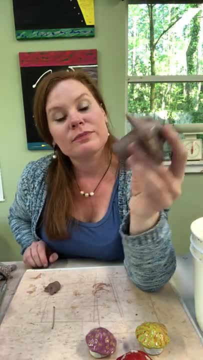 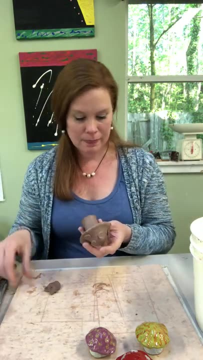 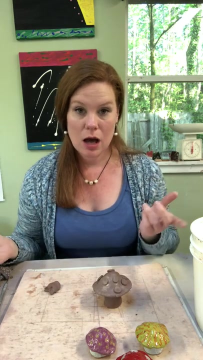 there's my little mushroom. um, yeah, he's still got his underneath designs. I messed, I squished a few of them, but I can fix them. so that's what we're doing. I can't wait to see what you come up with. you can leave me comments.